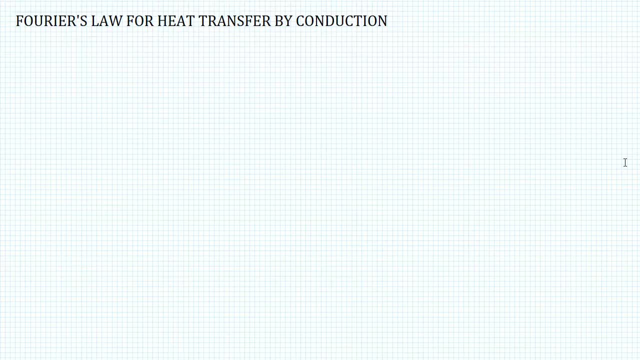 Conduction is a heat transfer mechanism that is crucial to a lot of unit operations. It's the result of transfer of vibrational energy between molecules in solids and of kinetic energy in fluids. Also, the movement of free electrons causes conduction, which explains why metals have such high thermal conductivity. 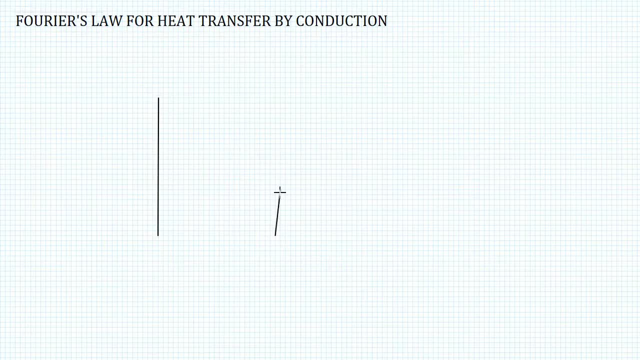 If we consider this plane wall through which heat is conducted. so the arrow Q represents the heat. the wall material has a thermal conductivity K and the thickness of the wall is X. Now heat transfer is happening because the two sides of the wall have different temperatures. 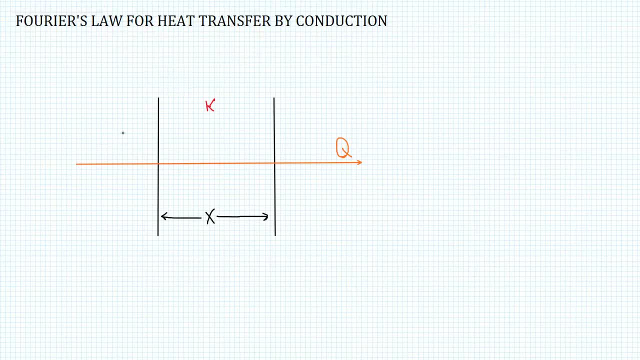 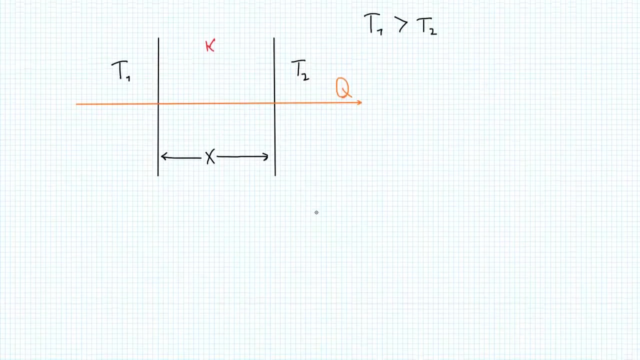 So we call one T1 and the other T2, and what this means is that T1 is higher than T2.. Fourier's equation explains this process. Fourier's equation explains this process of heat transfer by conduction by saying that the rate of heat flow Q. 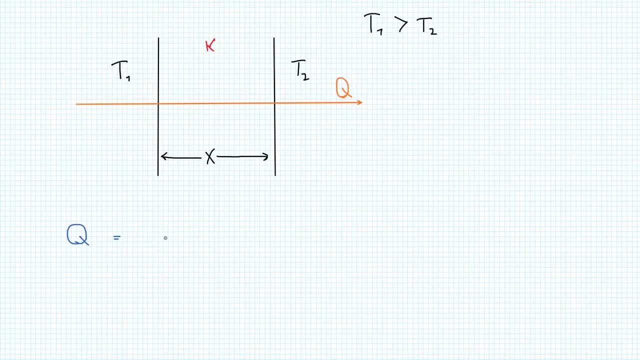 over the area A that we put on the right-hand side is proportional to the thermal conductivity K and the temperature gradient over the distance X, so dt over dx, which is the thickness, as we said before. So this is the simplest form of Fourier's law for conduction. 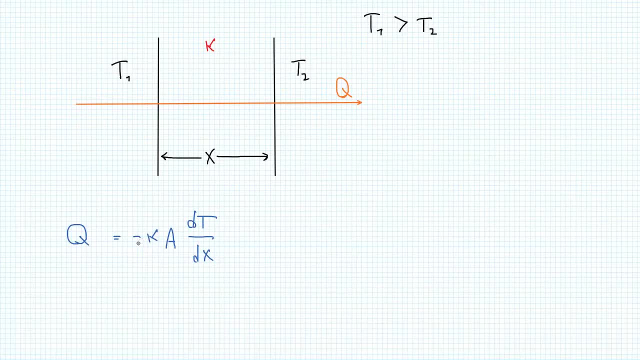 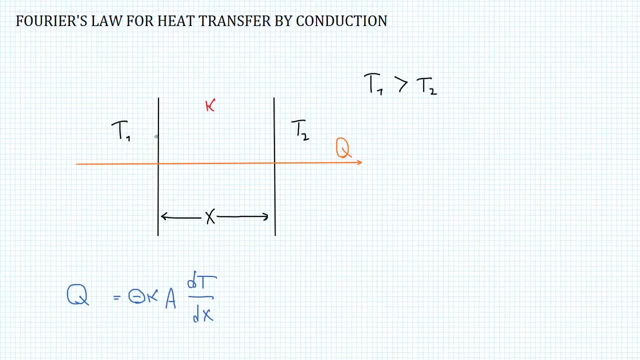 What's the negative sign there? That negative sign is there to take into account that the temperature gradient is in the opposite direction to the flow of heat. In fact, we can see temperature is actually decreasing as heat flows through the wall, which means that without that minus value, we always obtain values of heat flow negative. 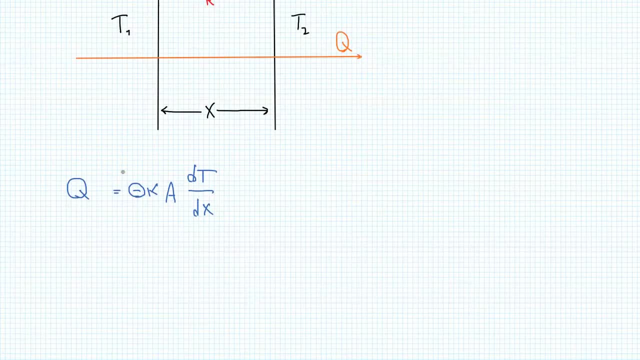 and so we put the minus to obtain positive values for Q. Applying Fourier's law to solve heat transfer problems involves identifying where conduction is actually happening. So in this case we know that the boundaries of the process are given by the thickness X. 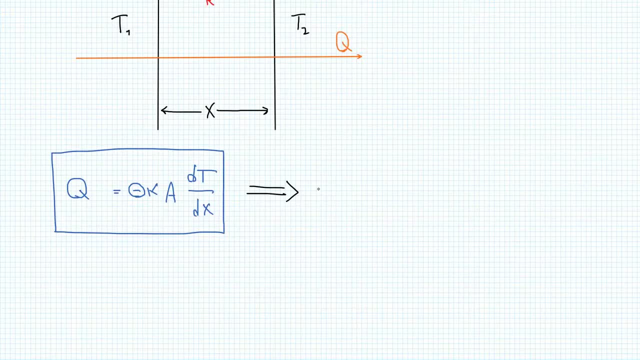 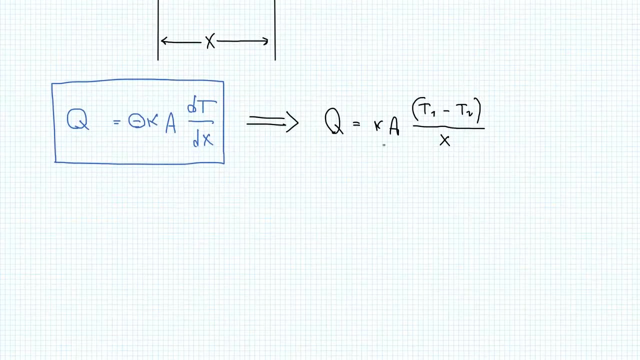 where temperature goes from T1 to T2.. So we'll integrate the equation for thickness X, obtaining that Q equals K times A over that delta T, with a negative sign in which then becomes T1 minus T2, over X. Often this equation is rearranged, bringing the thermal conductivity K to the denominator. 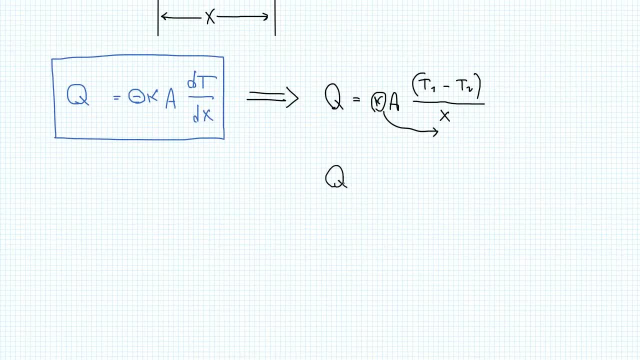 So the equation we'd be using is: Q equals A times T1 minus T2 over X over K, And this X over K is known as thermal resistance. It's a term that can often be found in problems specified as thermal resistance. Often the geometry of the system is not planar. 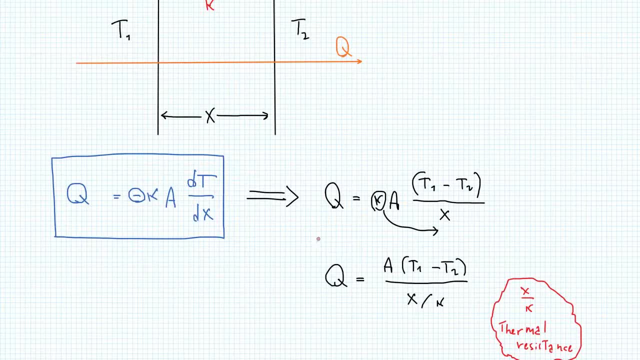 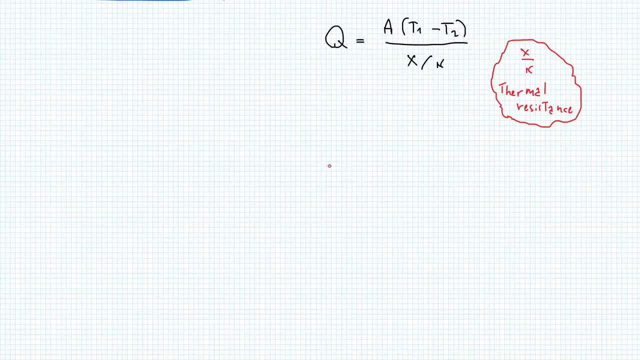 and the Fourier's law that we just looked at needs some adapting. For example, if you consider a tube, a thick-walled tube with temperatures inside and outside held constant, that would look something like this: We'll receive the section of the tube. 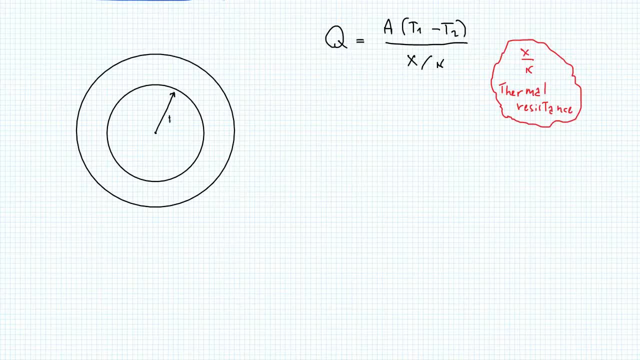 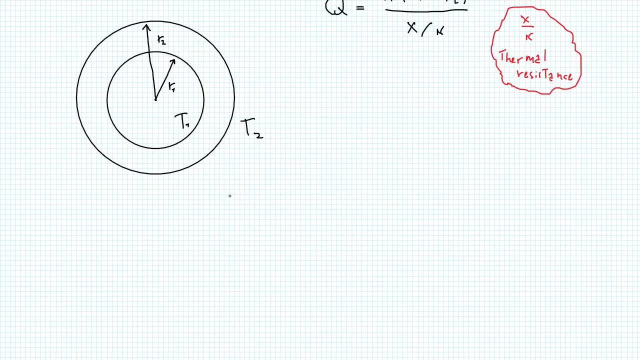 And the radii would be R1 and R2.. The temperatures would be T1 inside the tube and T2 outside, which would give us a direction of heat from T1 to T2, given that T1,, as we said before, is higher than T2.. 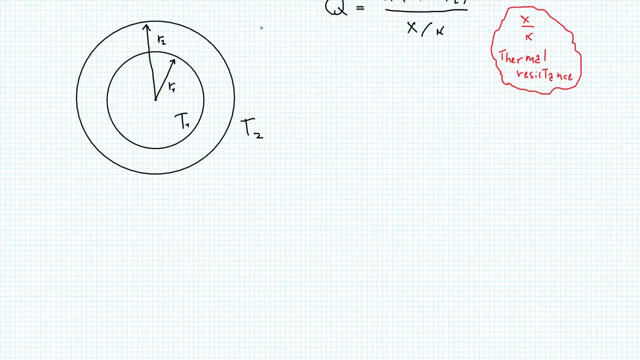 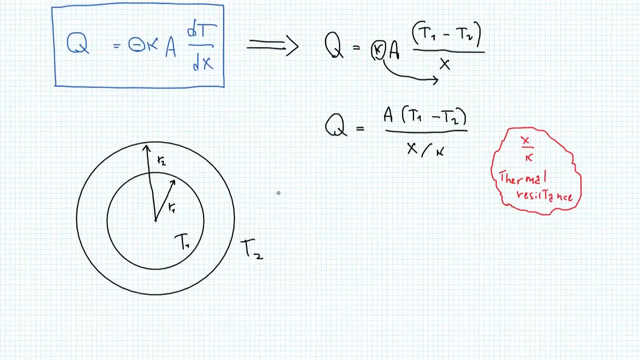 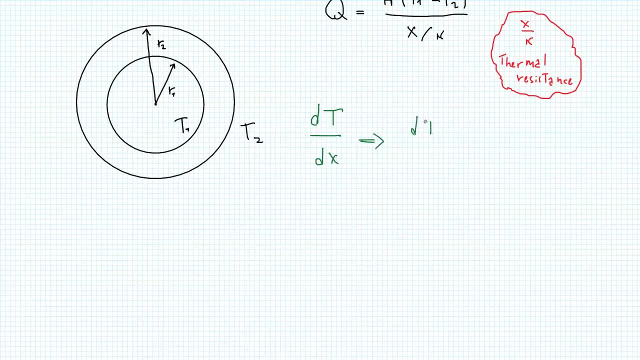 This type of geometries are better represented by polar coordinates As opposed to X and Y. Therefore, the temperature gradient that we looked at before, dt over dx, becomes dt over dr. The area available for heat flow would be the surface area of a tube. 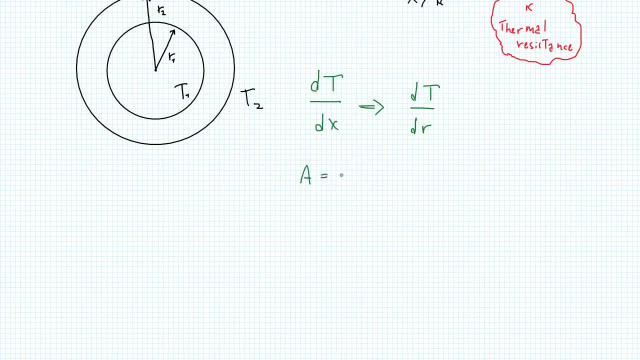 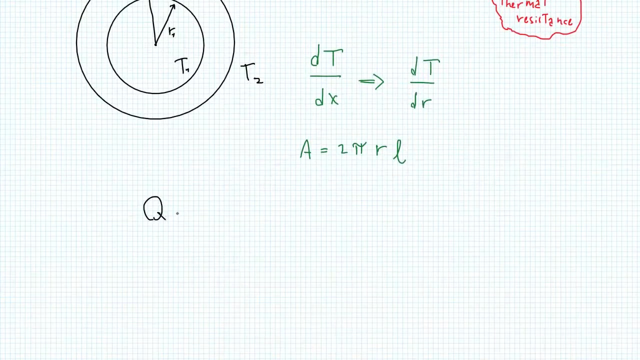 which is 2 pi r the diameter of a circumference times L the length of the tube. So putting together these considerations we get a version of Fourier's law. that's for conduction through walls of a tube, Q equals minus k, 2 pi rL times the temperature gradient, dt over dr. 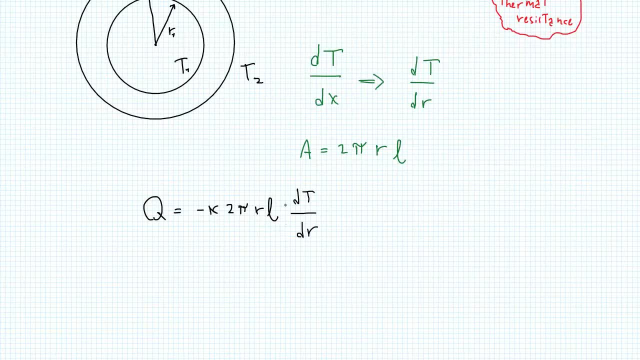 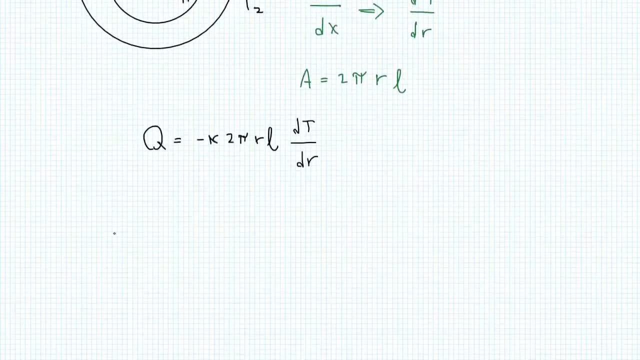 To apply this to solve heat transfer problems. we look at where conduction happens to find the boundaries for integration. So it's this red part between R1 and R2, where the temperature goes from R1 to R2.. From T1 to T2.. 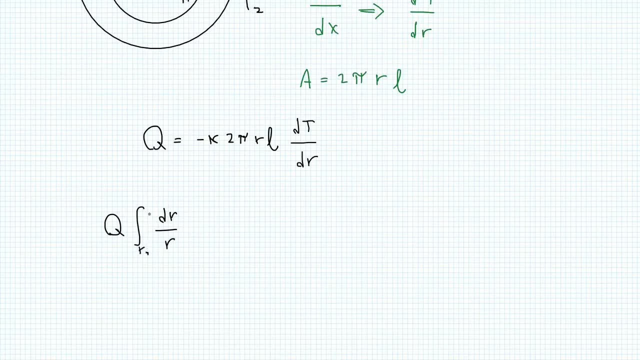 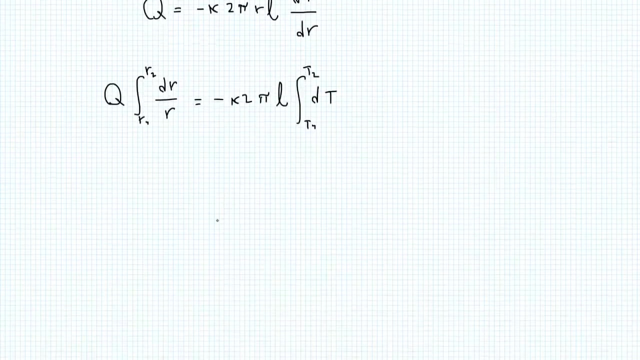 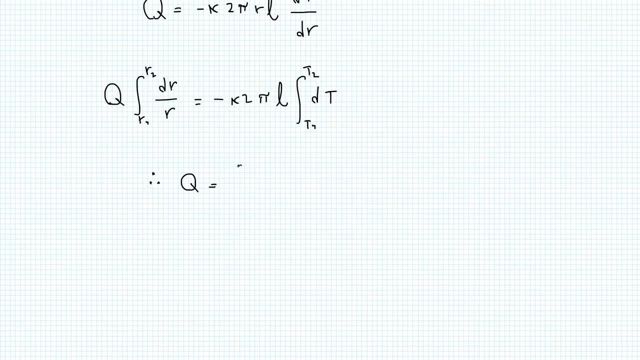 So Q times dr over r, that is integrated between R1 and R2, equals minus 2 pi Lk times the integral between T1 and T2 of just 1, dt Performing these integrals gives us an equation of Q being equal to 2 pi Lk times T1 minus T2. 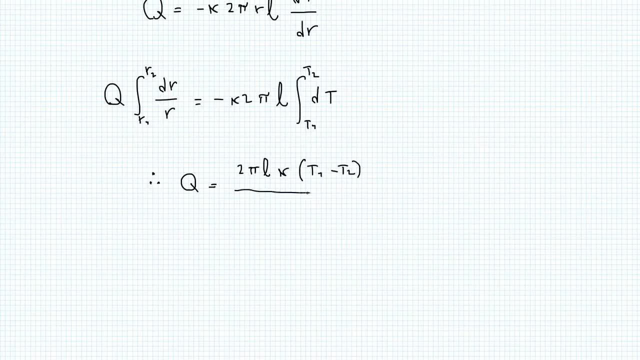 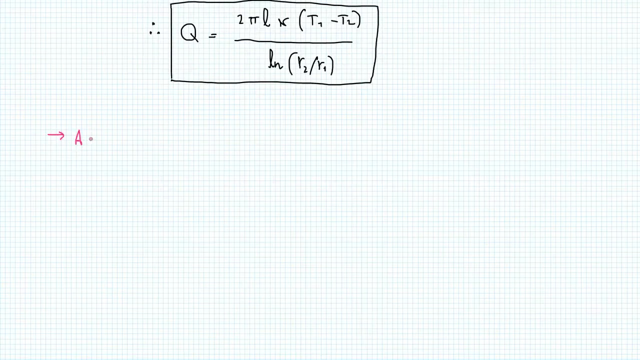 over the natural logarithm of R2 over R1.. So this is another form of Fourier's law. So this can be done in many different ways. This can be done in many different cases for other geometries to derive conduction equations, For example, a geometry where heat flows through the surface area of a sphere. 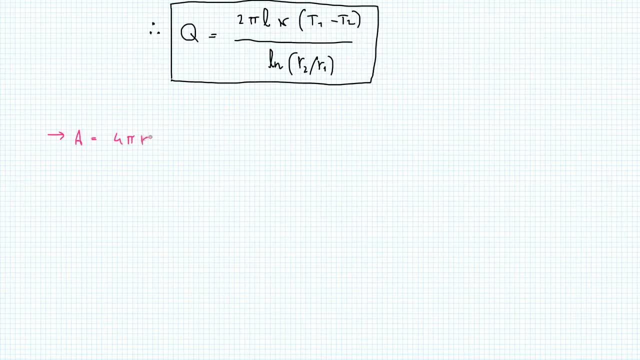 Well, in this case the area would be 4 pi r squared, meaning that Fourier's law would become: Q equals minus k, 4 pi r squared times the temperature gradient dt over dr, And, similarly as before, the conduction would be happening between R1 and R2.. 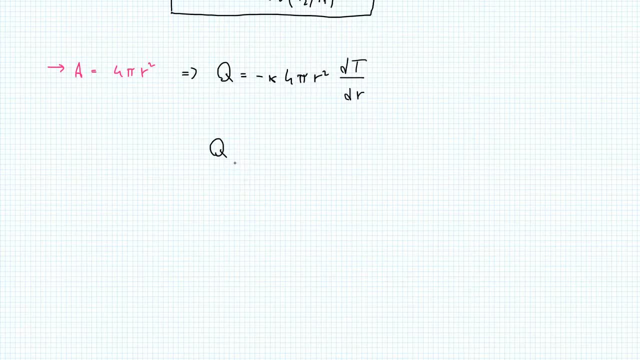 Therefore, the integration is between R1 and R2, where the temperature goes from T1 to T2.. And in this case the integrals would be of 1 over r, squared between R1 and R2 times Q, being equal to minus 4 pi k times dt. 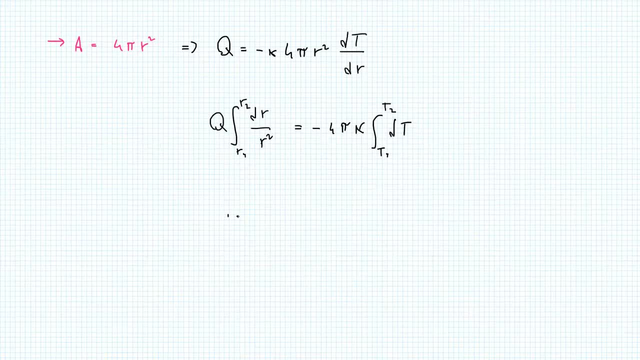 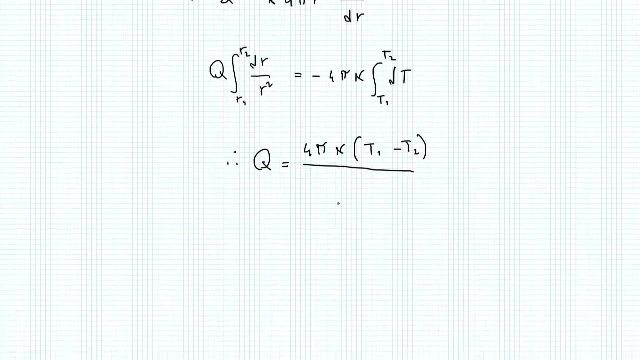 between T1 and T2.. So the integral of 1 over r, squared between R1 and R2, is minus 1 over r, giving us a final equation being: Q equals 4 pi k times T1 minus T2, and that's over 1 over r1.